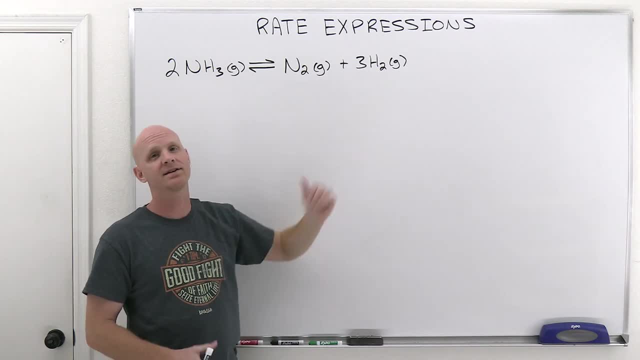 to do is first start looking at the rate of the reaction. So we're going to start looking at the rates of these individual reactants and products And we're going to start with N2.. And I'm going to actually give that to you, I'm going to tell you the rate at which. 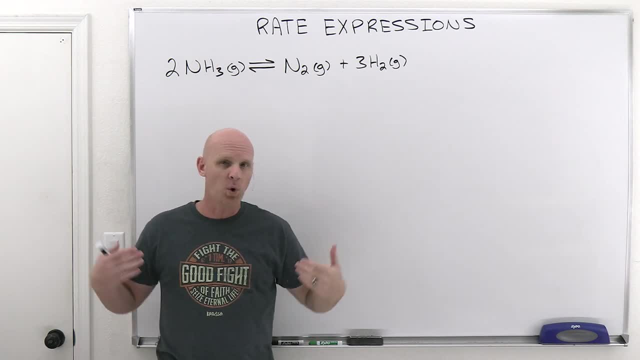 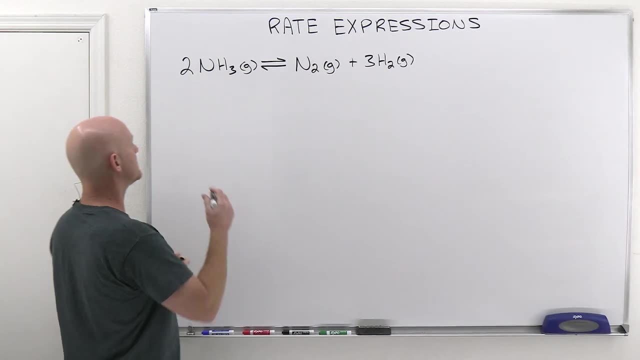 N2 is being produced in this reaction, let's just say, is 0.1 molar per second, And I could have given you you know it's going to have units of concentration per time. In fact, if we take a look, we'd often measure this rate as change in the concentration of N2. 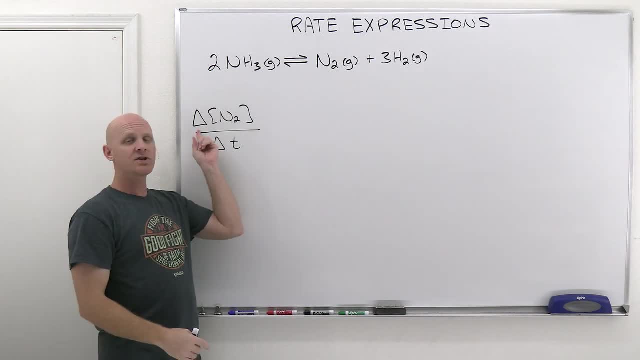 over change in time, And so anytime you look at that change, just remember that's final initial. So delta N2 here will be final concentration of N2 minus initial concentration of N2, and then change in time is just passive time: T final minus T initial, But since T initial 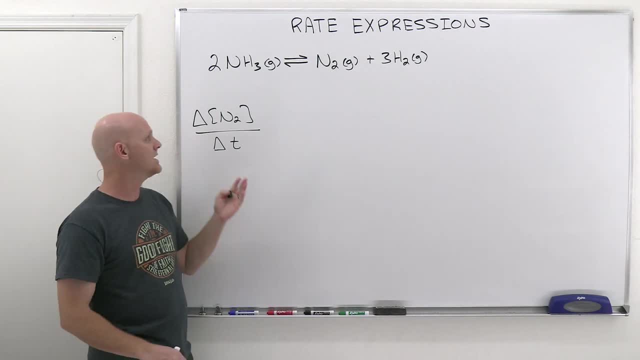 is usually zero, it's usually just whatever duration of time we're talking about, And so this rate here is expressed in units of molarity over time And that could be, like you know, molarity per minute, molarity per second. So those are the most common And 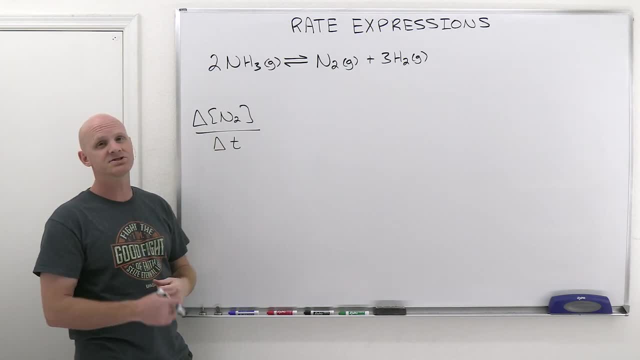 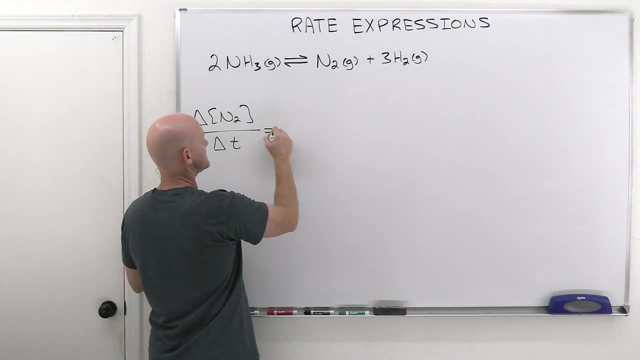 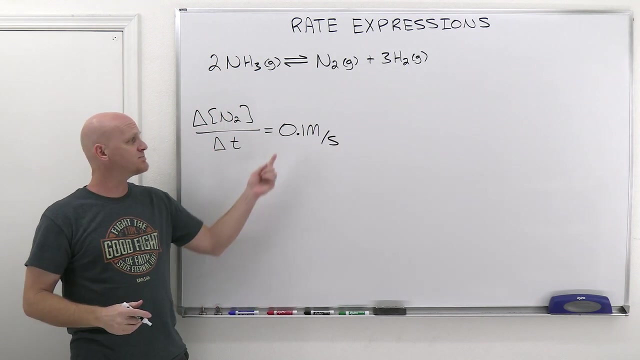 technically it doesn't have to be molarity, but it's going to be exclusively in this chapter, But you could have other units of concentration, So, but our brackets here definitely mean molarity, molarity, And so in this case I've told you that the rate here, in this case, is 0.1 molar per second. 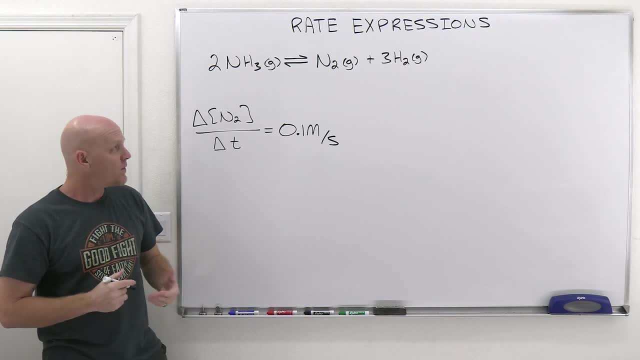 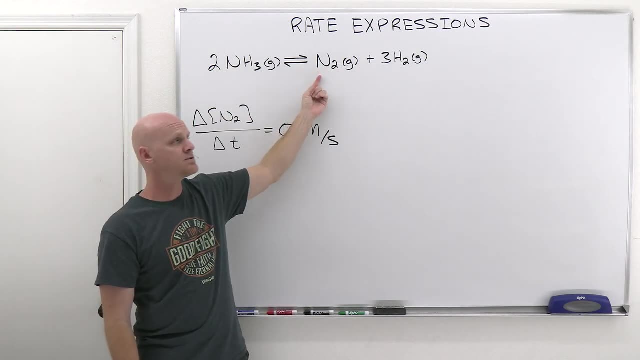 at which N2 is being produced, And so my question for you is going to be: well, what is the rate at which H2 is being produced? Well, we see that for every one mole of N2 being produced, we're going. 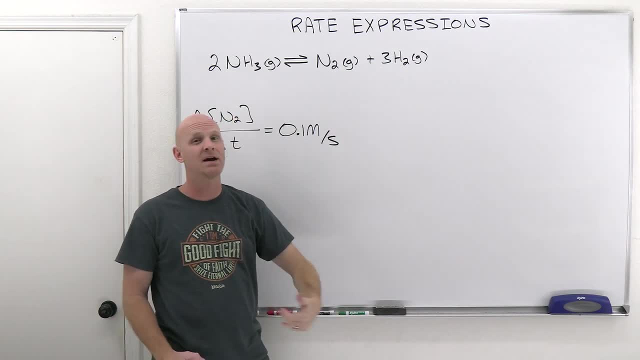 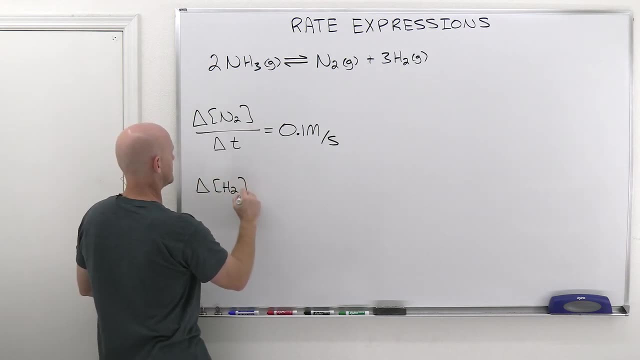 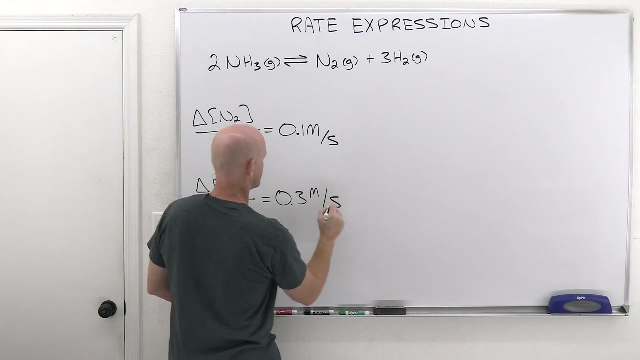 to produce three moles of H2, three times as many, which means it should have triple the rate. And so if we take a look at the change in the concentration of H2 over the change in time, that should be triple that number, so 0.3 molar per second. And then if we go back and take a 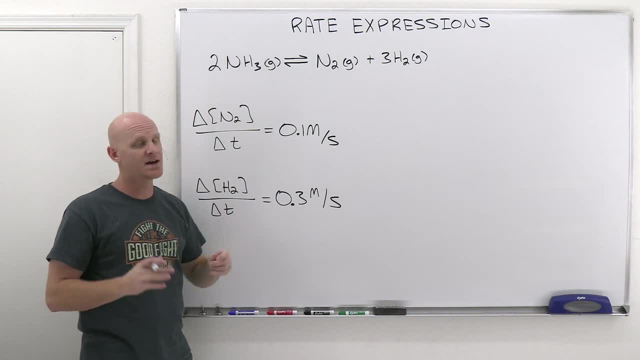 look at the rate at which NH3 is being used up here in this case, and again we're just going to look at the rate of change, though that'll be important here in a second. So we'll take a look at that change in the concentration of ammonia over the change in time And what we're going to. 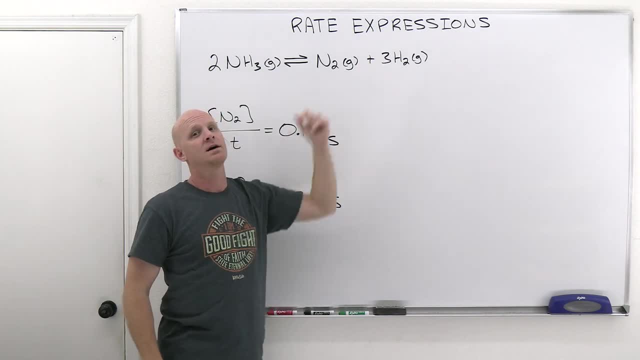 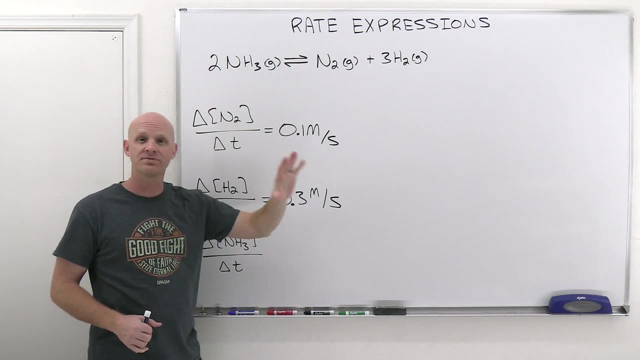 find out is that, whereas product concentrations go up- and when you have an increase, that's associated with a positive change- but reactant concentrations are going to go down as they're being consumed, And if you do final minus initial, you'll find out that that decrease corresponds to a negative change. And so 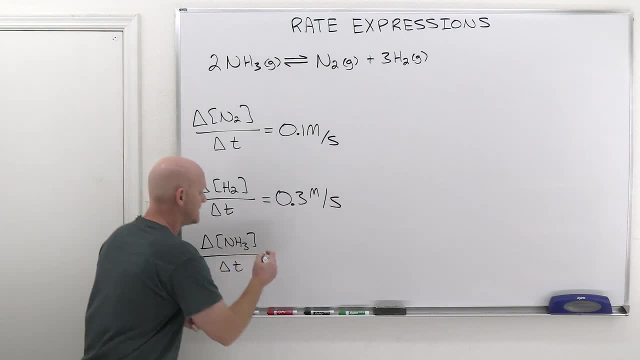 for a reactant here. this change in concentration over change in time is actually going to come out to a negative number. Cool. Now, in this case, we can see again that for every one mole of N2 being produced, we're going to consume two moles of NH3, twice as many, And so we're going to have a 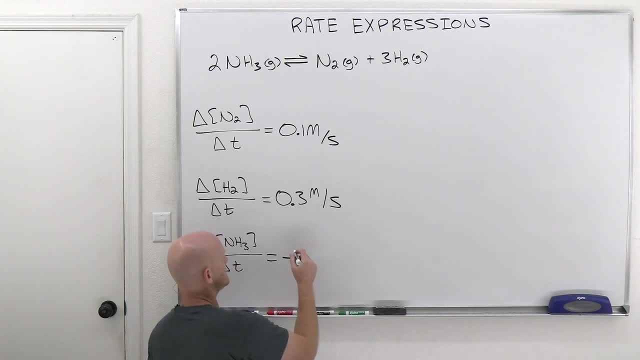 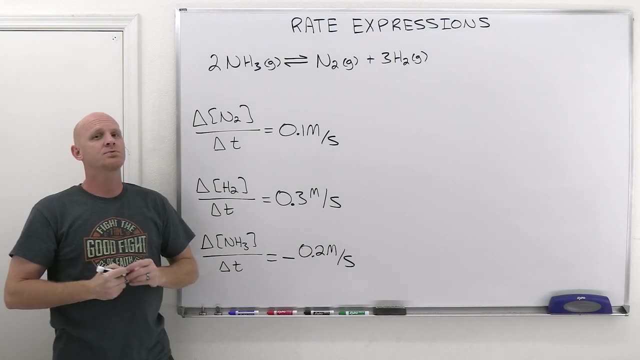 more effective rate of reaction, And so its rate's going to be twice as big as that of N2. And so in this case it'll be 0.2 molar per second. Cool, So now we've got three different rates here, one for 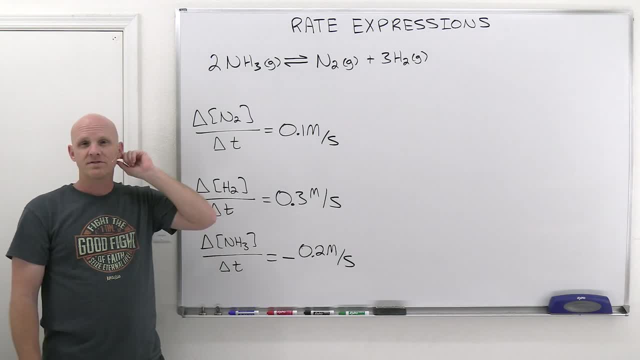 N2, one for H2, one for NH3.. So, however, there's something called the rate of reaction. So, and there's only one rate of reaction, not three, And so we got to figure out what is this rate of? 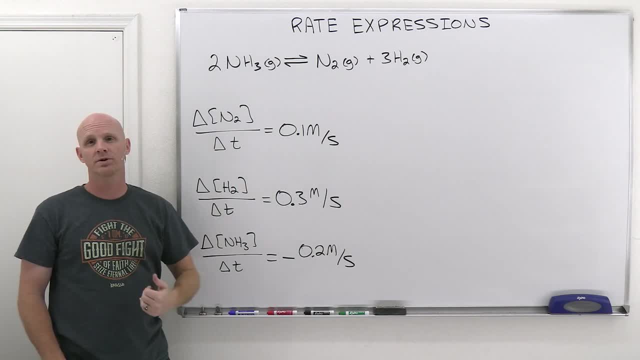 reaction. Well, it turns out, this rate of reaction is 0.1 molar per second. But how do we get that there and why is it that way, and things of this sort. and so it turns out that rates of reaction are always positive. so you should first know that they're not negative. so, and the rate of reaction? 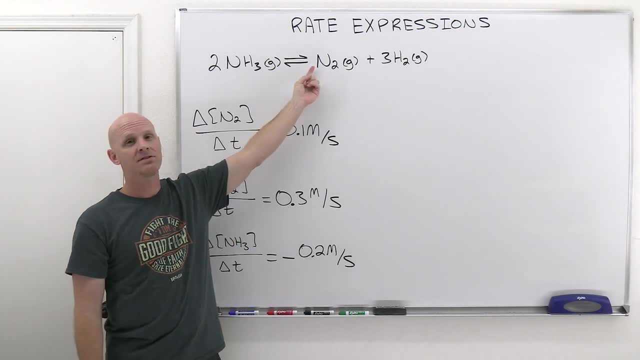 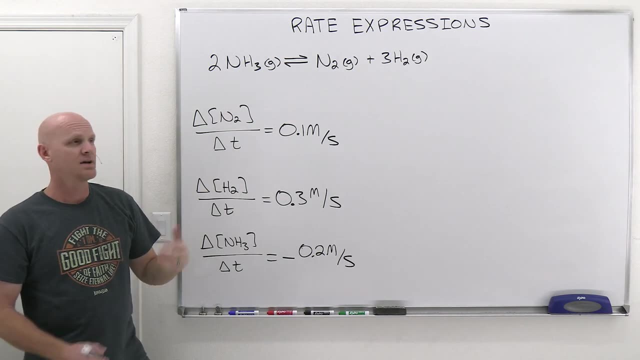 is essentially going to be whatever the rate for anything on the product side that has a coefficient of one, and that's why it ends up matching what it is for the case of n2. and so if we look, these rates of reaction, you actually get these from these rate expressions, and so in this case we 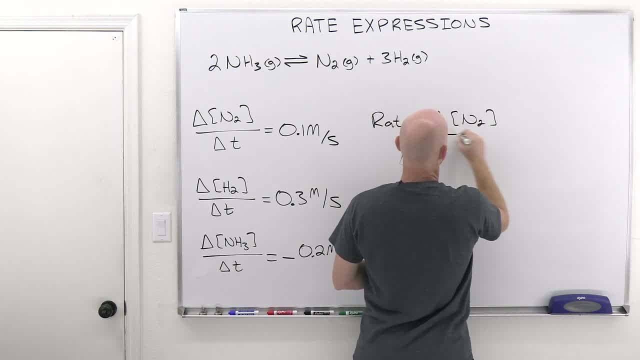 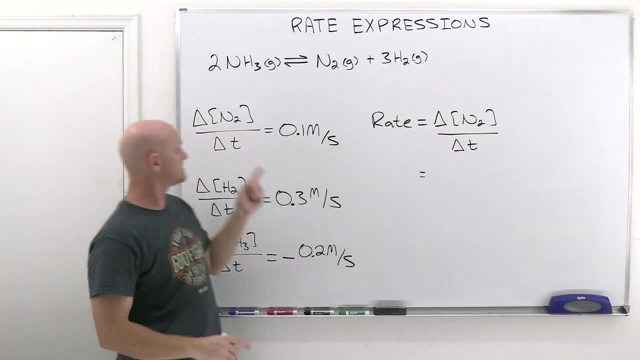 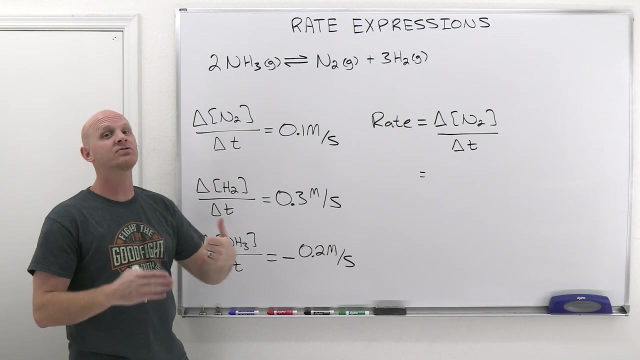 could have the change in n2 over the change in time, and that would be what we call a valid rate expression. if you calculate this out just like we was given here in this case, it will give you the rate of the reaction. it's not only the rate of change for n2 over time, it's the rate of the. 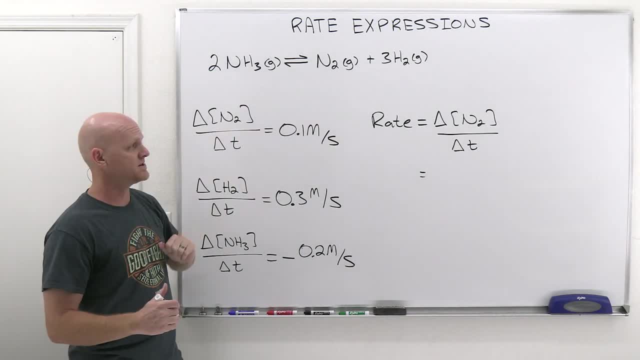 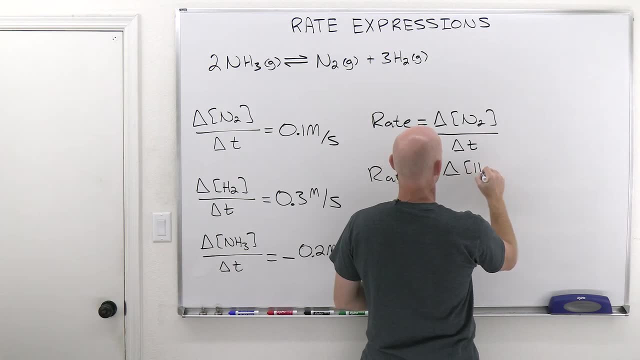 reaction. we say so, it's, more formally, the rate of the entire reaction. now if we try to do the same thing here again for the change in n2 h2 over the change in time, well, that's not going to be equal to the rate of reaction. 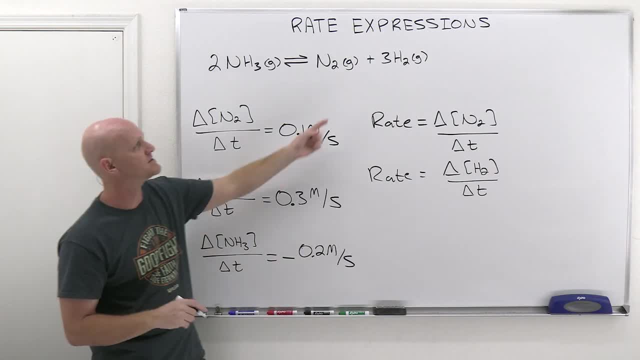 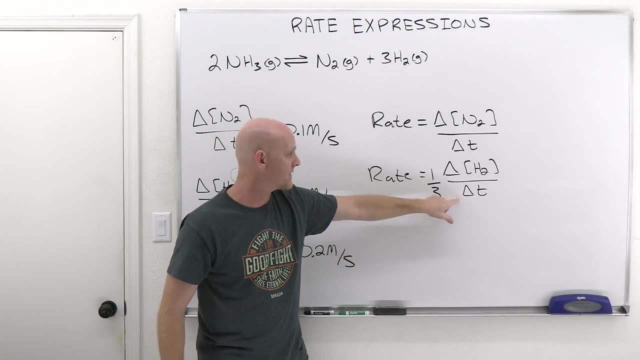 it's three times bigger, and so what you've got to do is you actually got to divide by that coefficient, which oftentimes we just write as a fraction instead. so we could have just put a three in the denominator here, or just multiply by one third. same diff either way, and so notice. 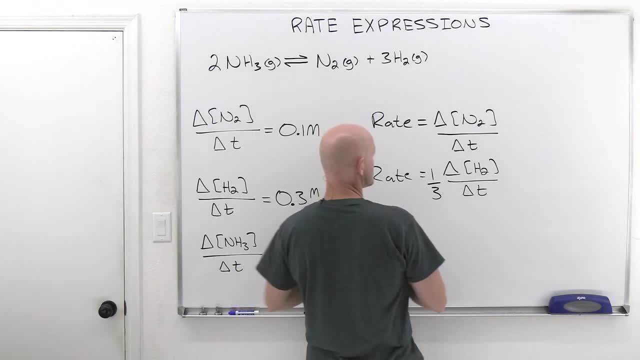 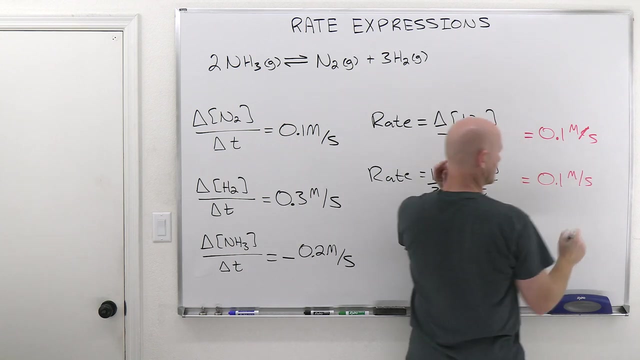 in this case, on the top example here, this would have come out to 0.1 molar per second and in this case- notice- it's going to be one-third times 0.3 and it's still going to come out to 0.1 molar per second. 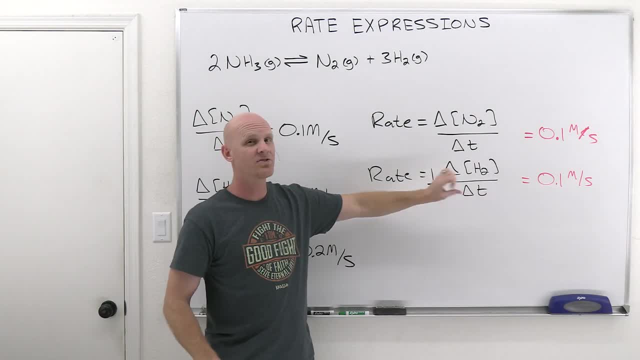 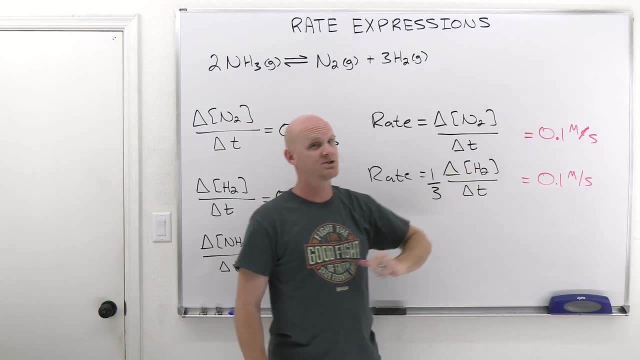 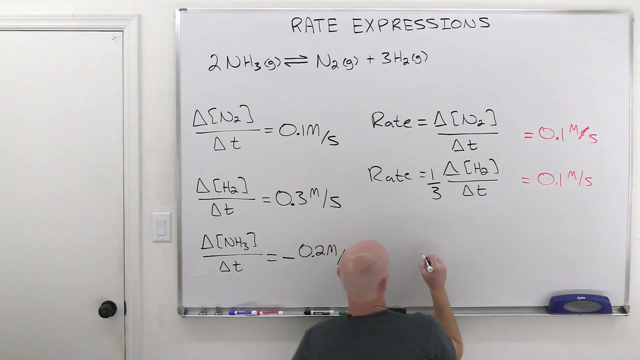 cool, so that's why it's a valid rate expression. these rate expressions take the rate of an individual reactant or product so and convert it by some factor into an overall rate of reaction, which is always the same. all right, so moving on here with nh3, and once again, if we just 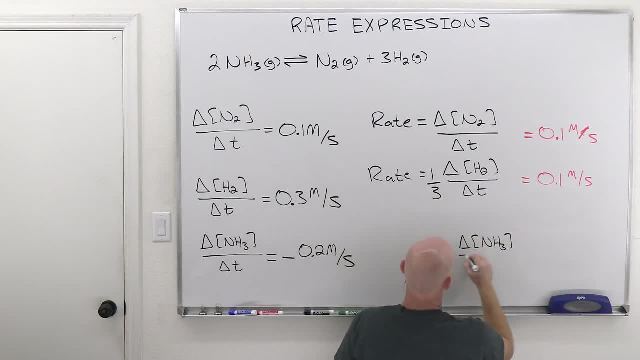 had change in the concentration of the reaction, we would be able to calculate the rate of reaction of nh3 over the change in time. we'd end up again with this negative 0.2 molar per second. so first thing we got to do is put a negative sign in there. that way a negative times, a negative 0.2, is going. 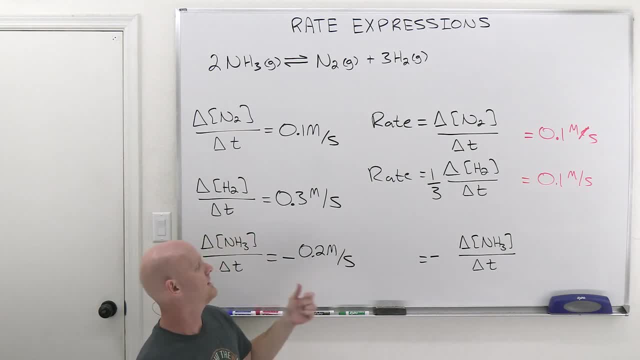 to come out to a positive number. and again, rates of reaction are always positive. the other thing we got to do is, again, once again, divide by the coefficient, in this case dividing by two, and again. whether i just put a two in the denominator down here or put a one half out in front, you'll see. 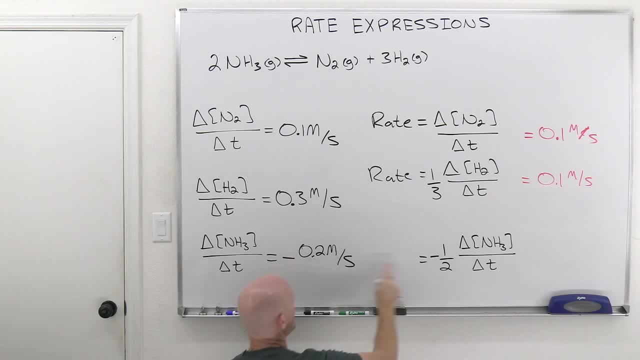 both. they're both customary. it means the same thing. and notice: negative one half times negative, 0.2 molar per second, because again, this is negative, 0.2 molar per second times negative one half is once again going to get us the same value here. 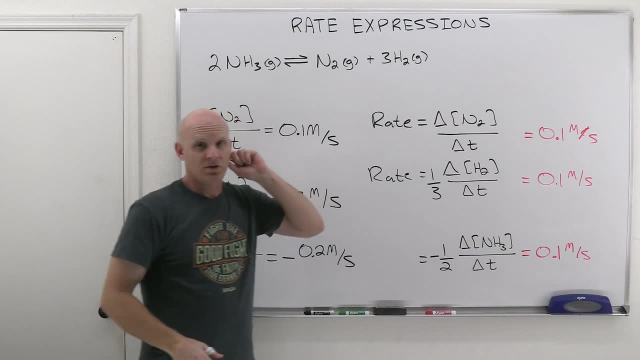 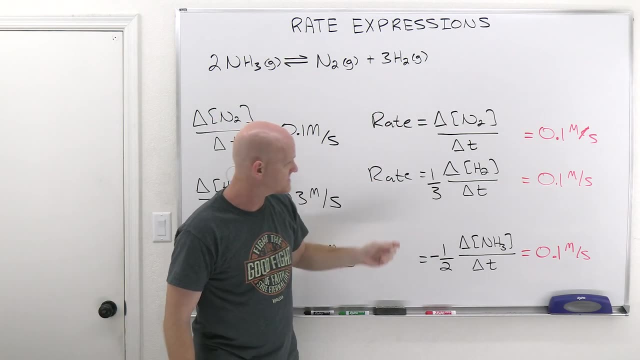 of 0.1 molar per second. so questions you might see on this of this order are: what is a valid rate expression for this reaction? and any one of these three expressions, including these fractions here, would be the valid rate expressions. the students don't often realize what they mean. 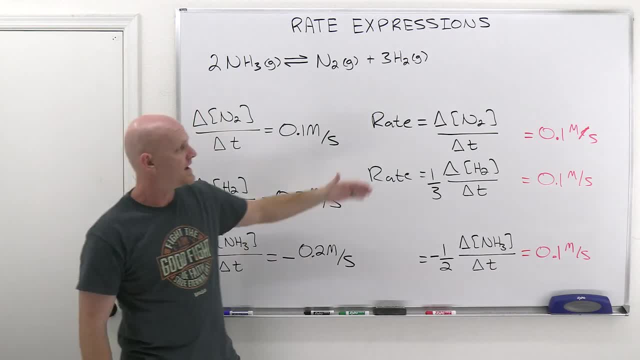 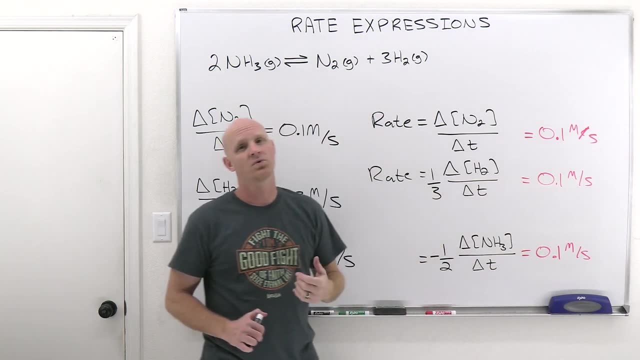 they just memorize. that's what a rate expression looks like. but the key is they take any reactants or products, change in concentration over change in time and converts it into the overall rate of reaction. that's what a rate expression accomplishes. so, if you get any, 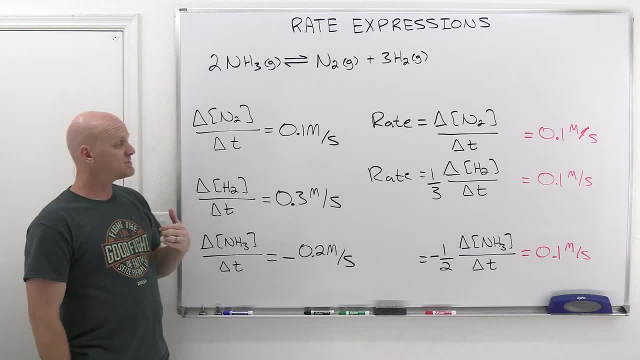 individual reactant or product and you're given one of the rates, you should be able to find the others. like we did here we took, i gave you the 0.1 molar per second for n2 over time and then we've translated that and figured out what the change in h2 over time or change in h3 over time would be. 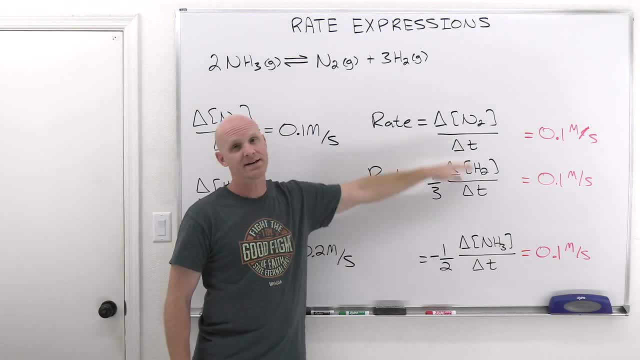 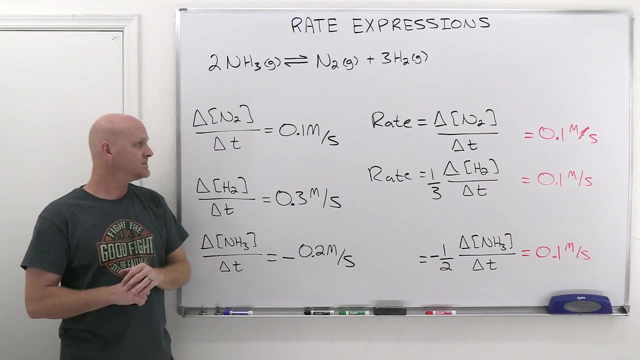 as well. so you should be able to do that, you should be able to determine any valid rate expression as well and find the overall rate of reaction. and one last thing i just want to give you here so that you'll be very careful. so if again for this reaction based on all the data i've got up, 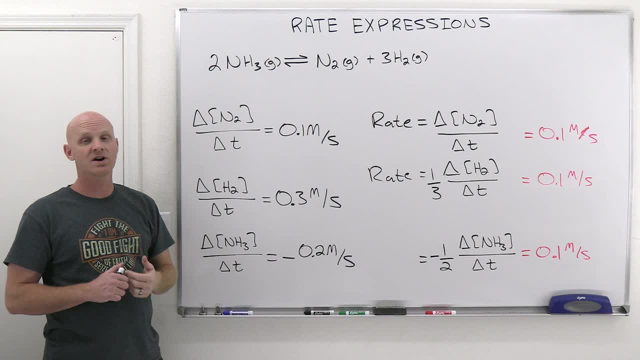 here if i said: what is the change? uh, what is the? the change of the concentration of n2 over time? 0.1 molar per second. so if i said: what is the rate at which n2 is being produced? 0.1 molar per second. 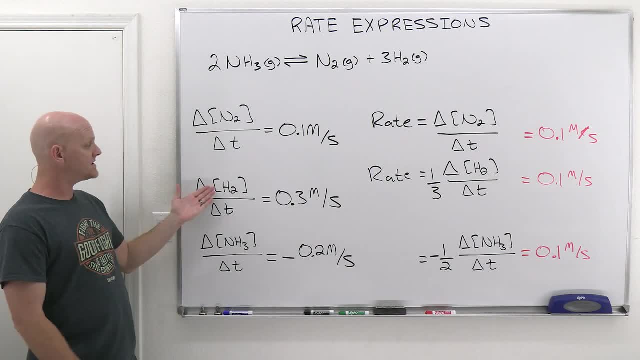 if i said what is the rate of change or the rate of production for h2 would be 0.3 molar per second. but for reactants you've got to be very careful. if i said what is the rate of change for the concentration of nh3 over time, it would be. 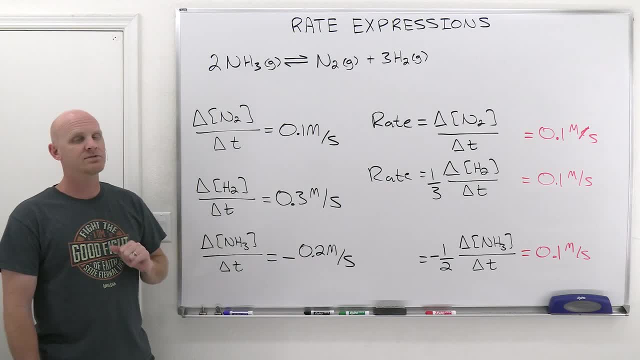 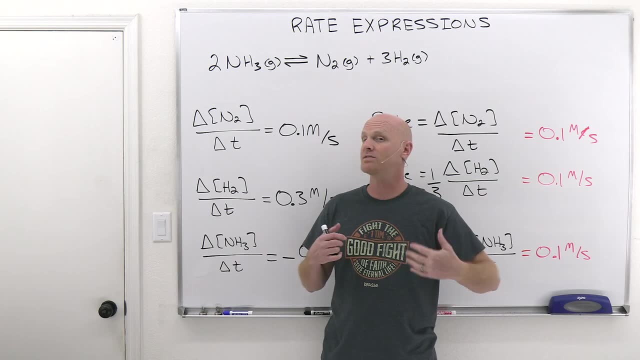 negative 0.2 molar per second. but what if, instead of saying the rate of change, what if i said the rate of consumption? and this is where you've got to be careful. if i say rate of consumption, that means i already know that that concentration is going down, it's being consumed, it's being used up. 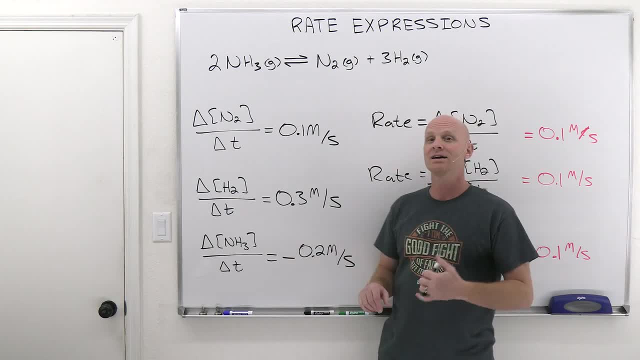 and so the rate of consumption is not negative: 0.2 molar per second, it's just 0.2 molar per second. so be careful for reactants. the rate of change is negative because if all i say is change, i don't know if it went up or went down. you need to tell me. but if i say rate of 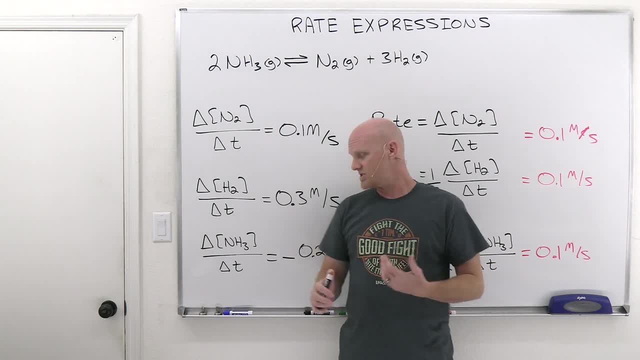 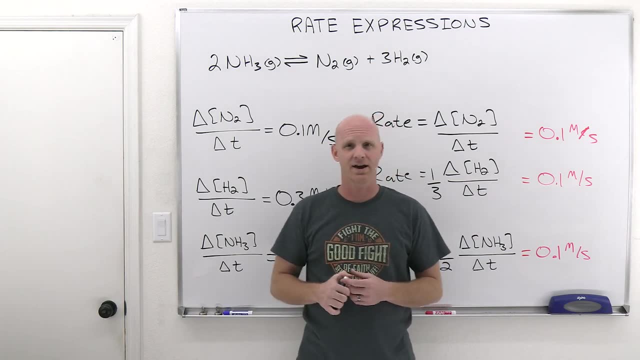 consumption. that's not the case. so you just give the overall absolute value of that number for reactants. so kind of look at it this way. let's say that, uh, you know, i know that you went to the casino on friday. so when i say, how did you do on monday? when you come back to you know class and 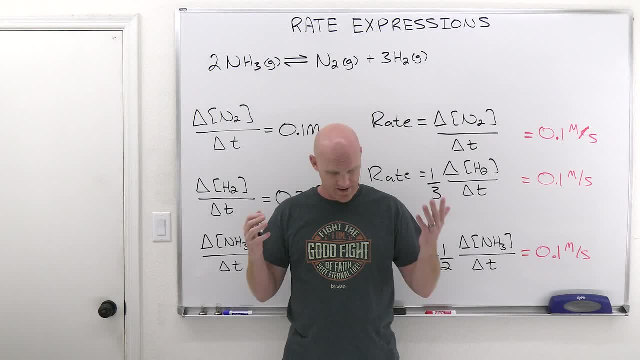 stuff and so and you say, hey, i lost 50 bucks. and i'm like, okay, you lost 50 bucks. and i said, no, no, i just want to know what's your rate of change and will you go? well, negative 50 bucks. so but if i know that you're a horrible poker player and there's no way you win because you? 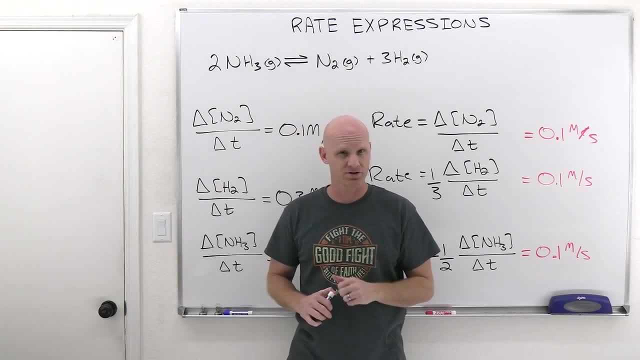 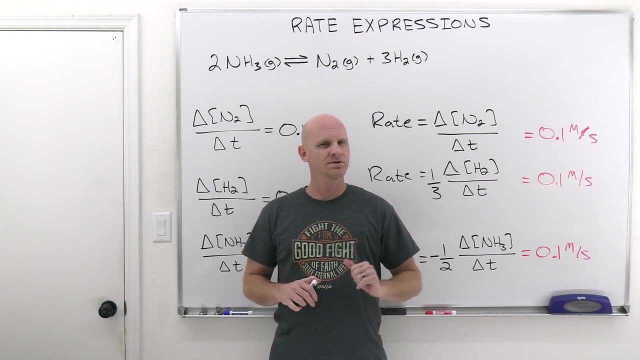 never win. and so, instead of saying how did you do or what's your rate of change, or something like this, i said: how much did you lose? are you gonna say negative 50 bucks, or are you just gonna say 50 bucks? because if i said how much do you lose and you say negative 50 bucks, i'm gonna be like 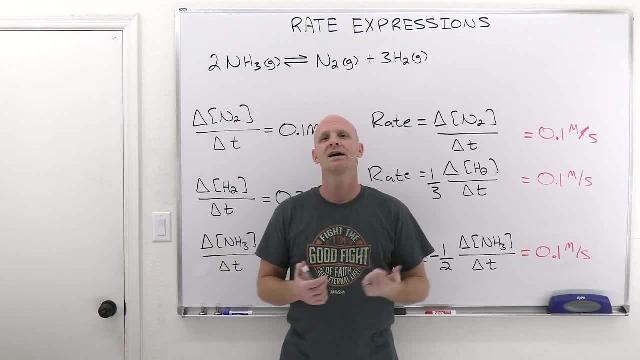 does that mean he gained 50 bucks? but you never win, you know. and so the idea is: when i say how much did you lose, i already know that your overall net worth went down. you don't have to tell me it's negative. i already know that it's implied in the question and you would just say: 50 bucks, not. 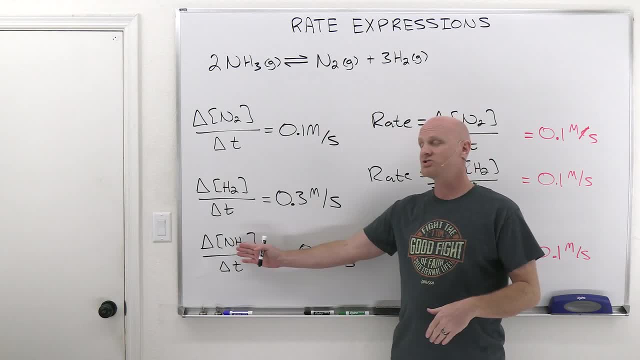 negative 50 bucks. that's the same thing going on here again. if i say rate of change for reactant, you better tell me it's negative. but if i say the rate at which it's consumed or the rate is which it's used up, then i already know it's going down and you're just going to give me the absolute. 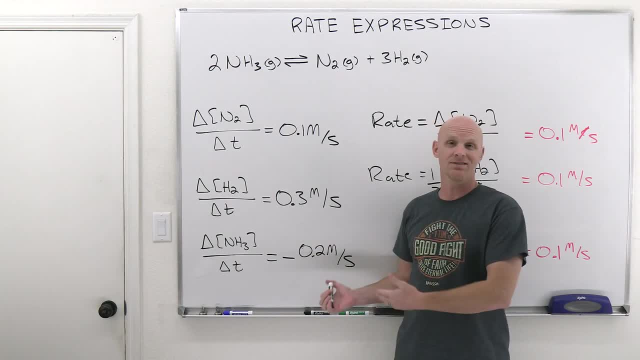 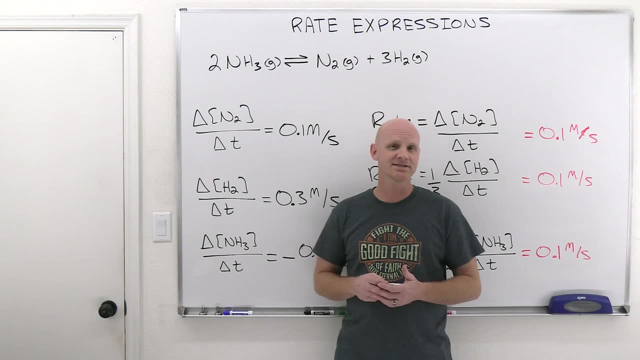 value of just plain old 0.2 molar per second in this case. now, if you found this lesson helpful, hit that thumbs up button. best thing you can do to let youtube know that other students need to see this lesson as well. and let me know in the comments below if you found this lesson helpful. 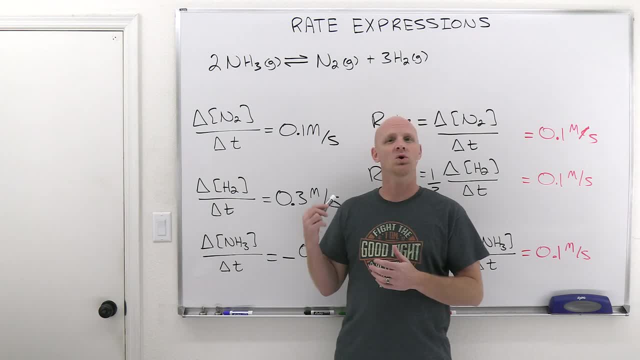 comment section what was helpful and if you've got any questions. i haven't quite cleared up in this lesson. now, if you're looking for the study guides that go with this lesson, if you are looking for practice materials on kinetics, check out my general chemistry master course. i'll leave. 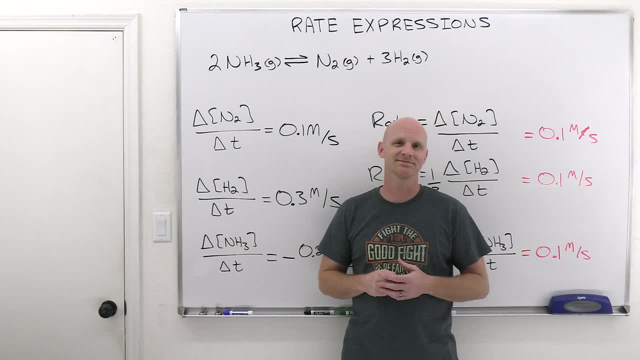 a link in the description, a free trial is available. happy studying. 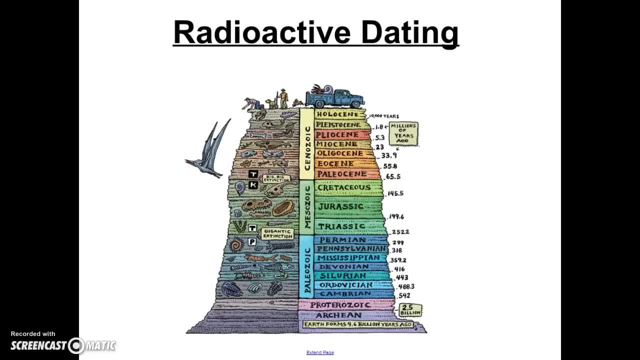 We've already learned how to determine the relative age of a rock or a fossil or a geologic event by comparing where it's found in relation to other objects. Today, we're going to take a look at how to determine the absolute age or the actual age of the object using a process. 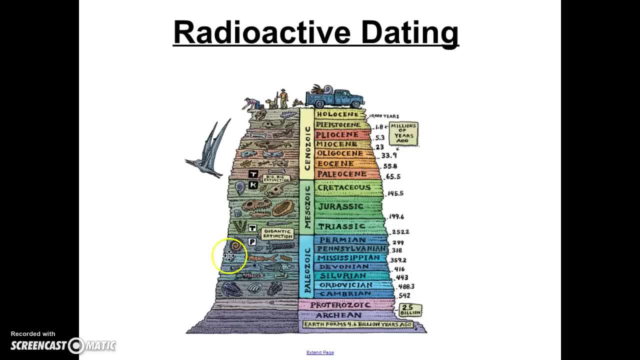 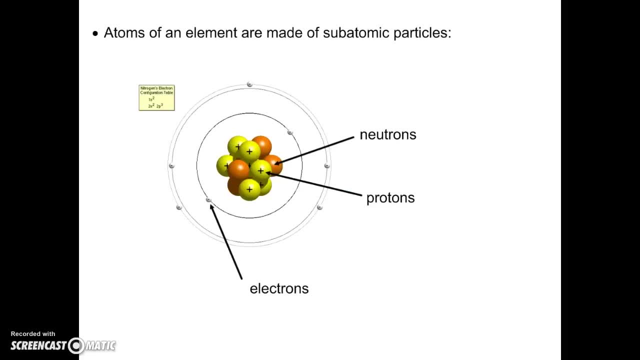 called radioactive dating. So let's say, you found a fossil and you wanted to know exactly how long ago this creature died. That's what we're going to learn how to do right now. So this is all based a little bit on chemistry, because it has to do with elements and atoms. We know that all atoms